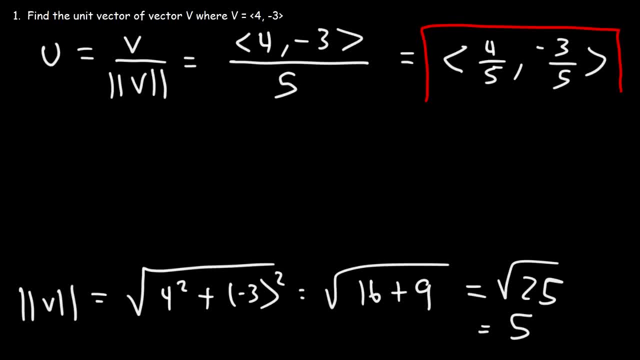 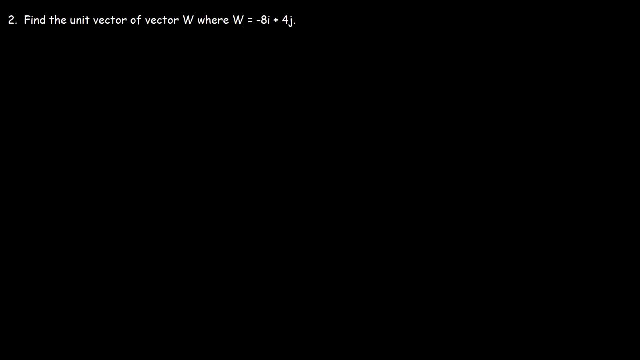 So that's a quick and simple way of finding the unit vector of another vector. Now let's try another example, One that's not so easy Like the last one. Feel free to pause the video and try this problem. So let's begin by calculating the magnitude of vector w. 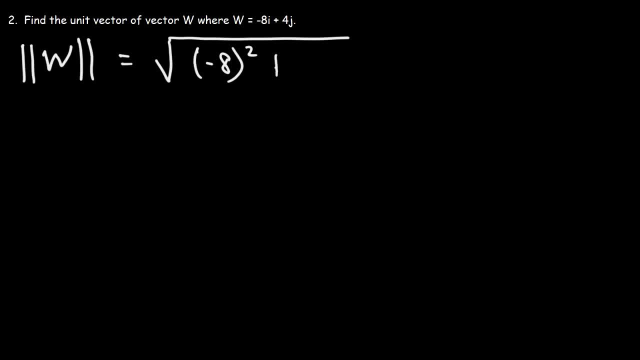 So that's going to be the square root of negative 8 squared plus 4 squared. Negative 8 squared is 64.. 4 squared is 16.. Now if we add 64 and 16, we're going to get a square root of negative 8 squared. 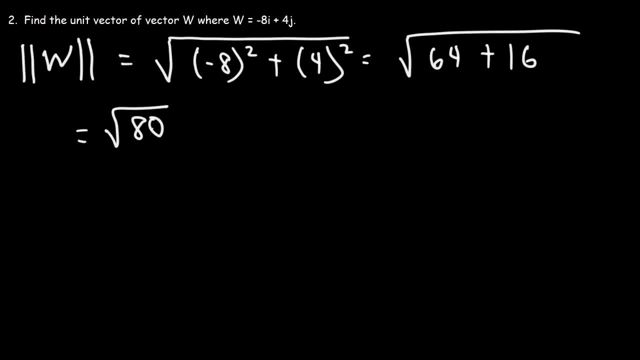 So we're going to add 64 and 16.. That's going to give us 80.. Now, 80 is not a perfect square, so we need to simplify the radical. So what two numbers can we break up? 80, one of which is a perfect square? 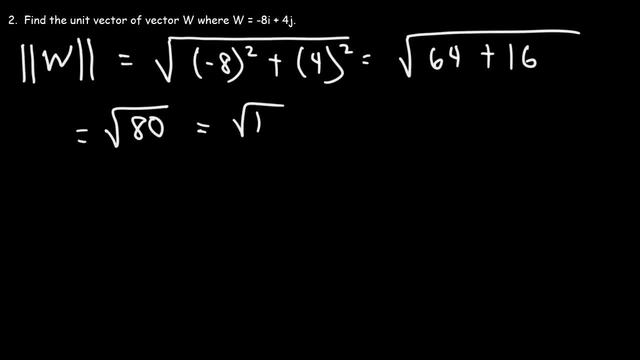 The highest perfect square that goes into 80 is 16.. If you divide 80 by 16, you get 5.. So we can write the square root of 80 as the square root of 16 times the square root of 5.. 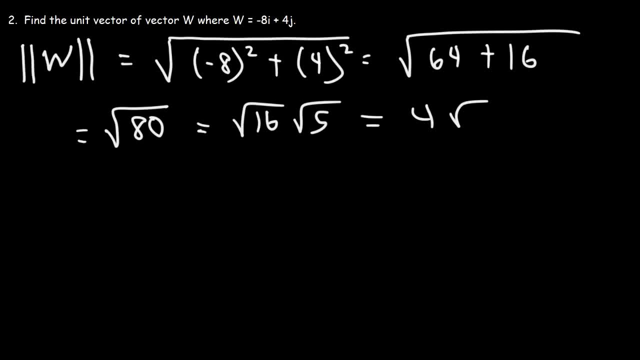 Now the square root of 16 is 4.. So now we have the magnitude in its simplified form. It's 4 square root 5.. Now let's determine the unit vector. So it's going to be vector w divided by the magnitude of the vector. 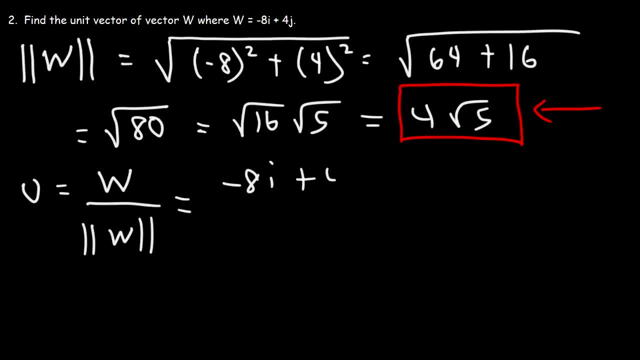 So w is negative 8i plus 4j, And we're going to divide that by 4 square root 5.. So now let's separate this into two fractions. So let's divide negative 8 by 4 square root 5.. 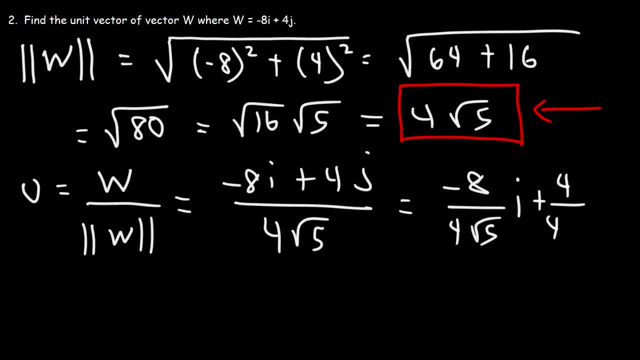 And then we're going to divide 4 by 4, square root 5. Negative 8 divided by 4 is negative 2. So we have negative 2 over square root 5 times the unit vector i. And then here the 4s cancel. 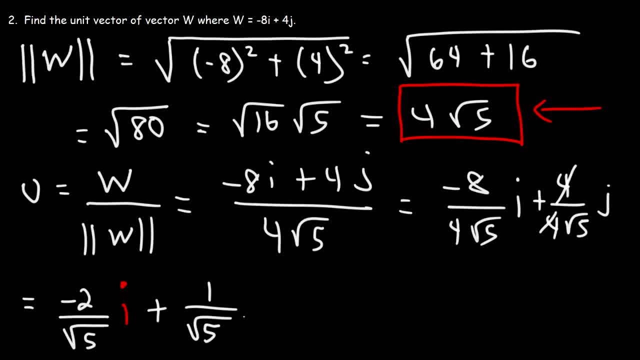 4 divided by 4 is 1.. So we get 1 over square root 5 times j. Now you can leave your answer like this if you want to. It is correct, but we could simplify further if you wish to rationalize the denominator.